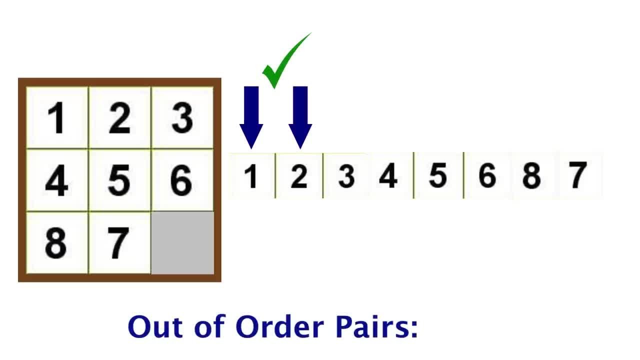 The 1 and the 2 are in order because 1 comes before 2, as it should. 1 and 3 are good. Even 1 and 8 are good because 1 comes before 8 numerically, as it should. 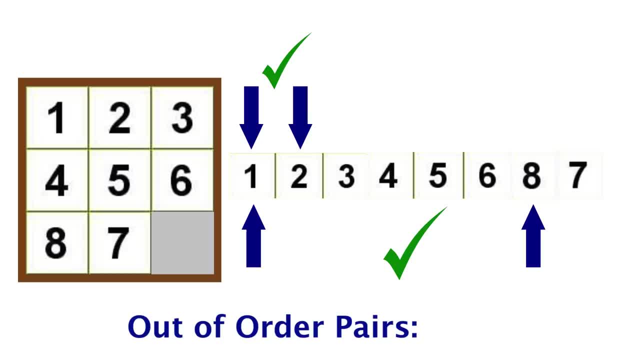 In fact, every pair of numbers is in relative order except 7 and 8. Thus we have one pair out of order. The goal is to have 0.. So now let's do another vertical move and move the 6 down. 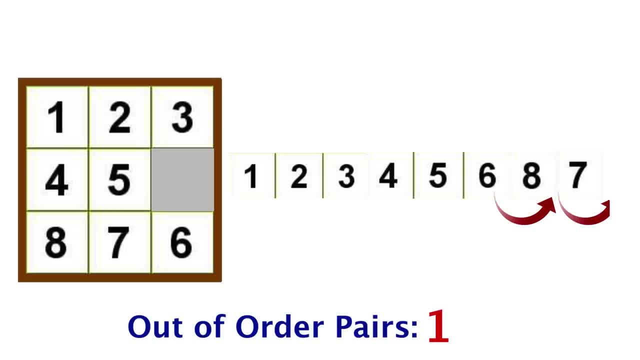 On our linear number line. we know the 6 moves two places to the right, But before I move it, look closely. Originally the 6 and the 8 are in order because 6 is supposed to come before 8.. 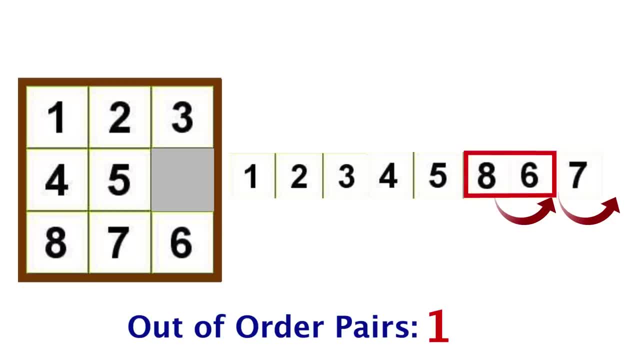 Once I move it, they are out of order and our out-of-order pairs changes from 1 to 8.. But of course we're moving it two spots. It was in order with the 7, but that changes as well, leaving us with 3 pairs out of order. 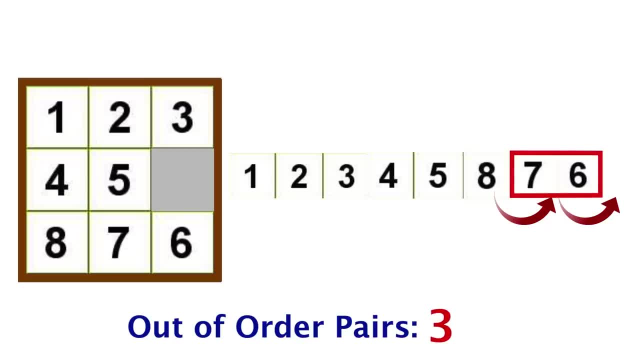 So we did a vertical move. the number moved two places backward, which changed our out-of-order pairs by 2.. 1 for each move. In fact, no matter what the order, every time a tile makes a single move along our number line. 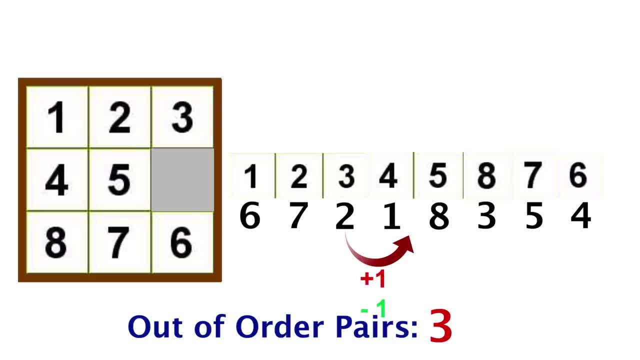 the out-of-order pairs will either increase by 1, or decrease by 1.. If the two numbers are out of order after a move, they will be in order. thus, however many out-of-order pairs we have will decrease by 1.. 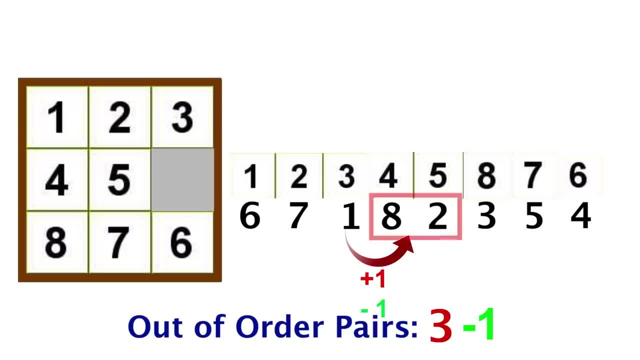 And if they're initially in order, after the move they will be out-of-order. thus, an increase in one. Each single move makes the out-of-order pairs either increase or decrease by 1.. But remember, when we move vertically, the only way to change the order of everything. 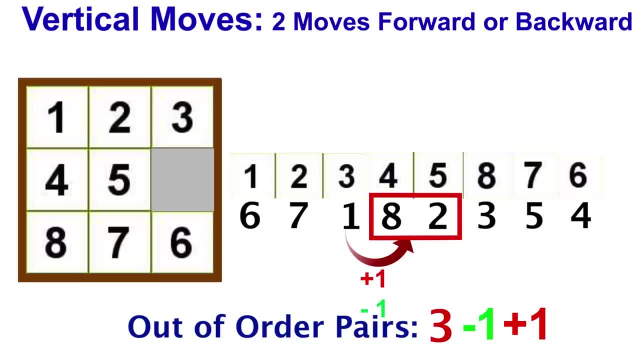 tiles move two places over-that's our only option. If each move either increases or decreases the out-of-order pairs by 1, then after two moves you can either have a a change of 2, a change of 0, however it may happen- or a decrease in 2.. This is all that. 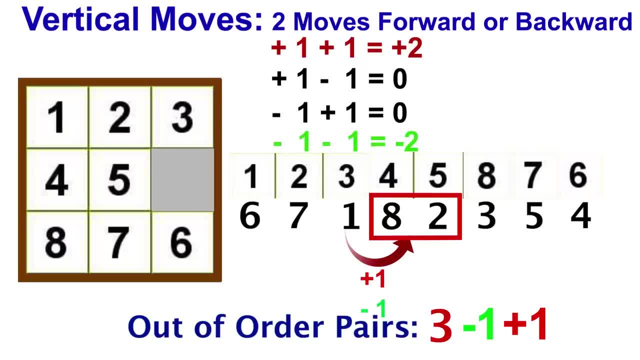 a vertical move can do If our puzzle starts with one out-of-order pair, and these are the only options. no matter how many moves we do- adding 2,, subtracting 2, or staying the same- there is no way to reach 0 out-of-order pairs, which was our goal. Thus this puzzle. 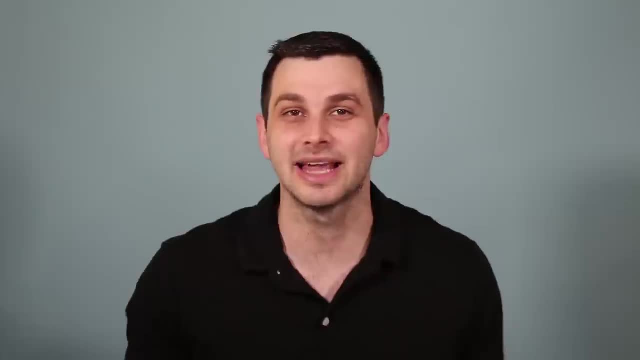 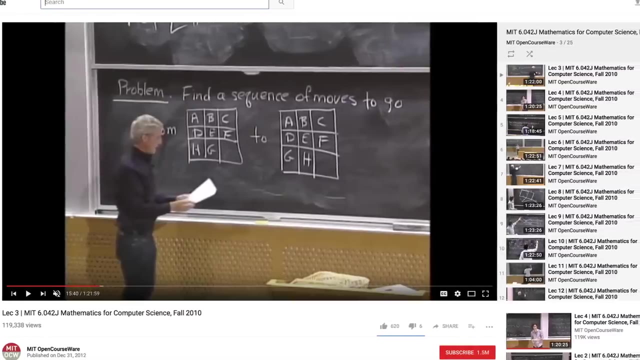 is impossible. Hopefully this wasn't too confusing, but I really like this example. This is a famous problem in discrete math and is even taught at MIT in their Mathematics for Computer Science class. I like this example because there was virtually no mathematical background. 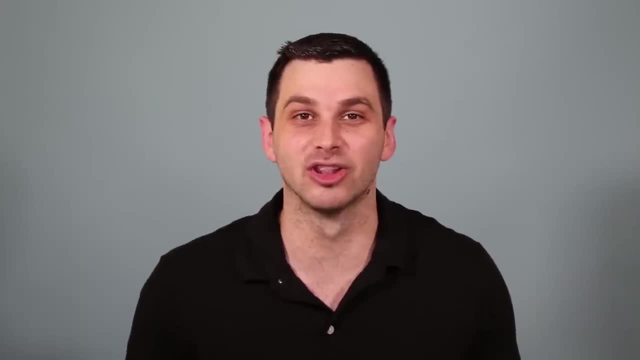 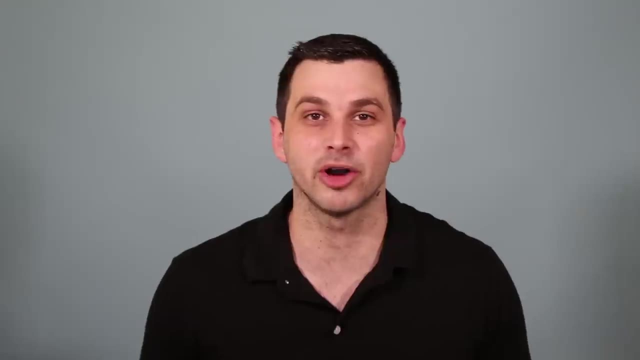 needed, but it did involve mathematical reasoning and I'm sure most people just can't look at it and understand it immediately. Computer scientists and mathematicians have to do proofs like this all the time to understand a system or model from the ground up, and I hope you. 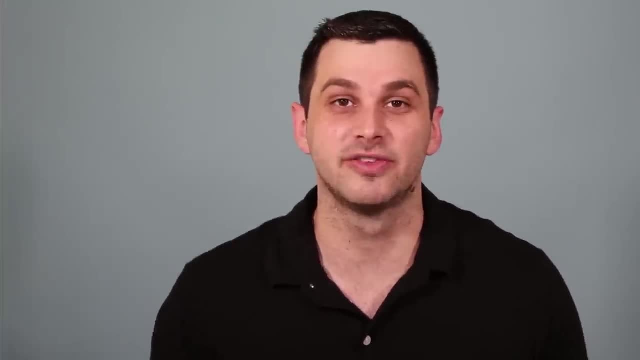 realize that it's very different than what you see in most high school math classes. This video is really on the mathematics that computer science and math majors see, as well as a few others, but I really wanted the focus to be on computer science and math, so I'm 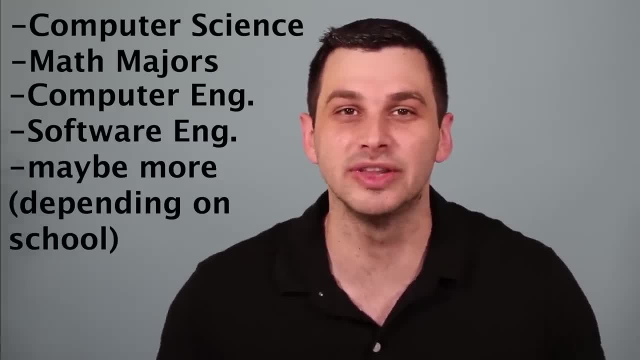 going to focus on computer science because, especially if you go into research, this is the kind of math you will need a foundation in. In this video and the next I will show applications, but the proofs won't be anything that a mathematician would approve of due. 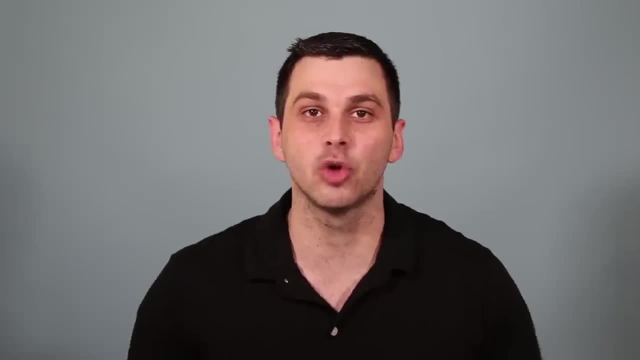 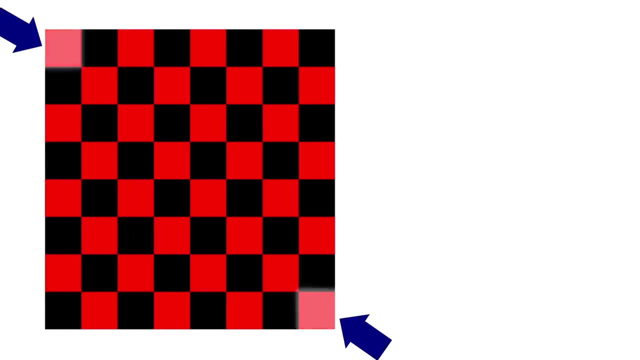 to time. Now let's go into another proof. that's much easier and, again, needs no real mathematical background, just logical reasoning. Let's say you have an 8x8 checkerboard with the end corners missing. The question is: can you fill up every space with 31 domino pieces? 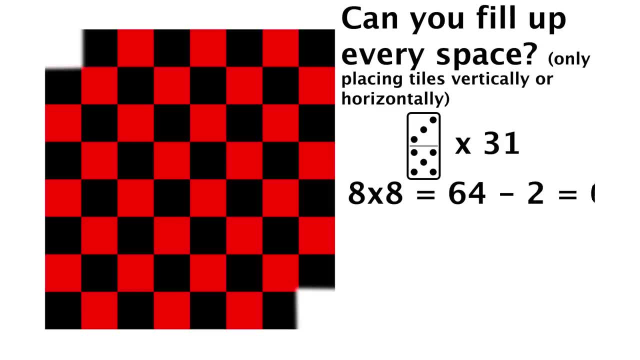 It has 64 squares minus 2 from the ends. missing is 62.. And 31 dominoes that cover 2 spaces each would cover a total of 62 spaces. But how can we show that it definitely is or is not possible to cover the entire board? See if you can get it, but the answer is fairly. 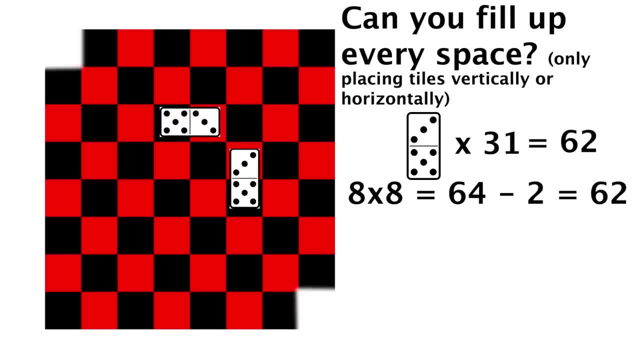 simple. Whether you orient the domino vertically or horizontally, it will cover one black space and one red space. Therefore, 31 dominoes would have to cover 31 red spaces and 31 black spaces. If you notice, those missing end pieces are both red, which means there are 32 black squares. 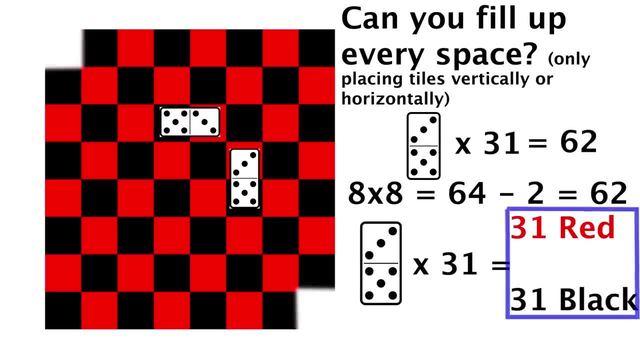 and 30 red squares. Like we said, we would have to have 31 of each and since we don't, there is no way to cover the entire checkerboard with these and our proof is done. These proofs are often the beginning of a discrete math class. You will learn proof. 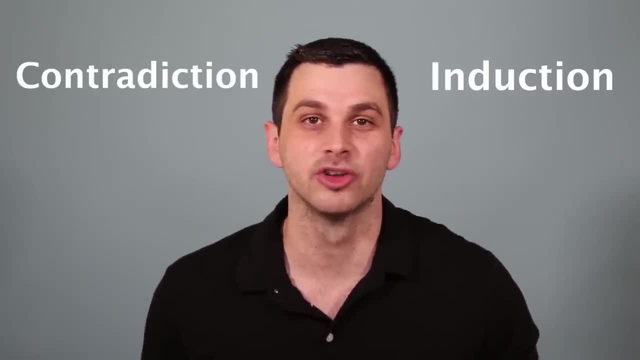 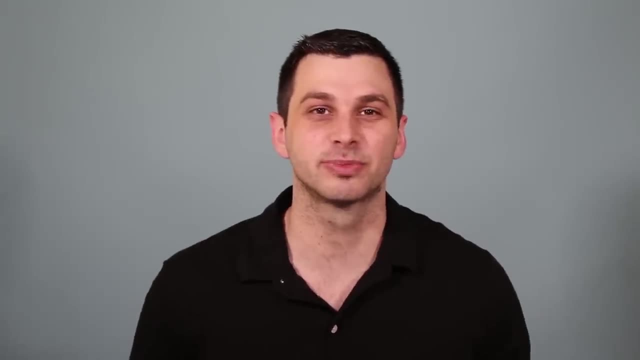 techniques like proof by induction or contradiction that I won't go over, so know, it's not just all puzzles like these. While these are more general examples that might not have a direct, obvious application, you have to learn these proofs so you can then apply them to the more applicable problems. 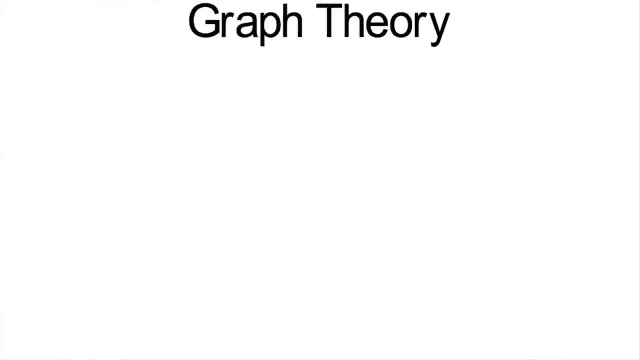 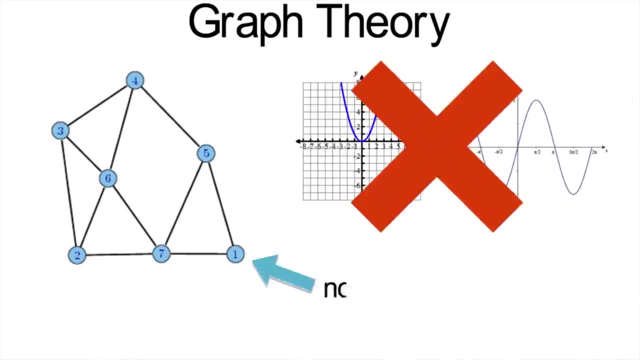 which I'm going to go into now, starting with graph theory. This is a huge field in math and computer science. In graph theory, graphs are not like x squared or sine of x. Graphs have a bunch of dots or nodes and lines that connect. 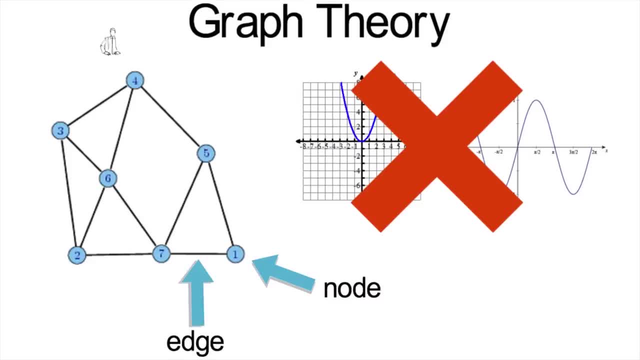 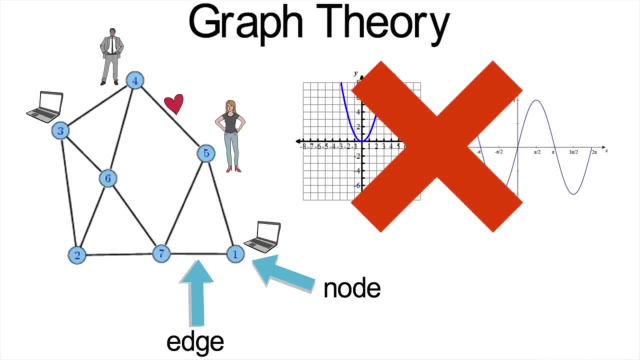 I'm going to show you how to do that in just a few minutes. I'm going to show you how to do that in just a few minutes. I'm going to show you how to do that in just a few minutes. Nodes could represent computers and the edges are cables that connect them where data needs. 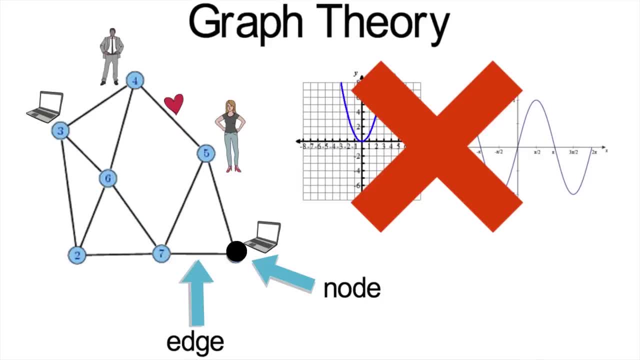 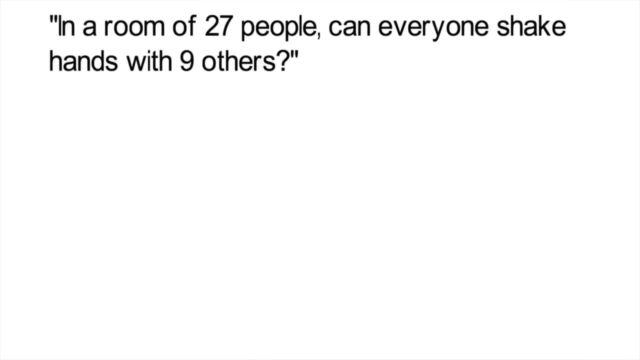 to travel the shortest path to reach its destination, Or nodes could represent destinations like cities, and edges are highways or roads that connect them. Many of these problems are not very easy, but here's a simple question you can use graph theory to solve. In a room of 27 people, can everyone shake hands with 9 others? 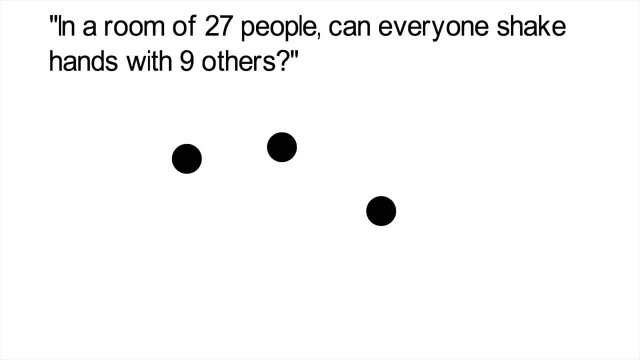 Well, since this is graph theory, we'd have 27 nodes which represent the people. I won't show all 27 dots, but here are some to illustrate the solution. Now, if a pair of people shake hands, we can represent that with an edge. 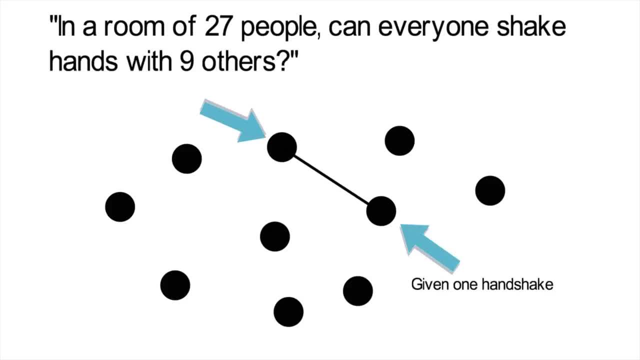 So right now, this person shook one person's hand, and so has this other person. The question is: can everyone shake hands with 9 others? To solve this, we only need one piece of background information. Look at this graph I just randomly found and count how many edges or lines leave this. 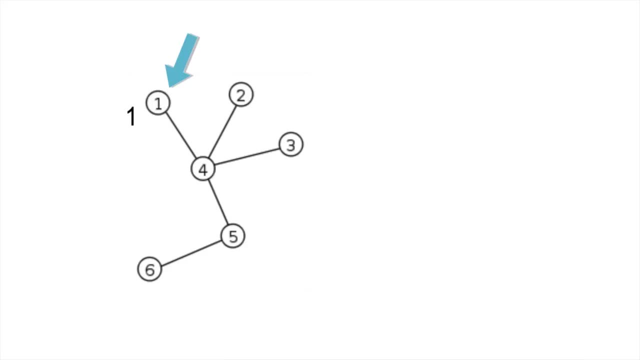 dot or node? Of course, there's only one. This is the degree of the node. Now, what about node 4?? Well, we see there are 4 edges leaving it, which is its degree. If we do this for every node, these are the amount of edges leaving each one, or the degrees. 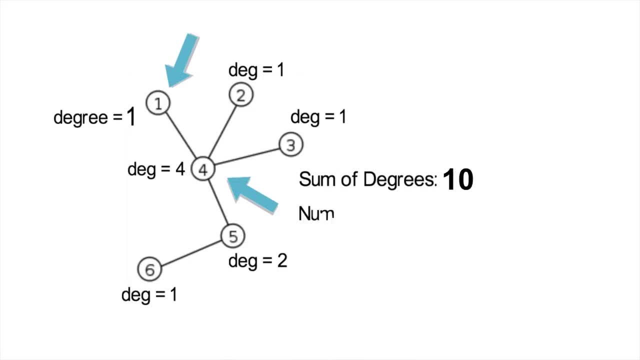 Add all these degrees up and we get 10.. Now that we have that, count the amount of edges or lines that you see. You'll find there are 5,, which is half the sum of the degrees. If we look closer, we'll see this is always the same number of edges or lines. 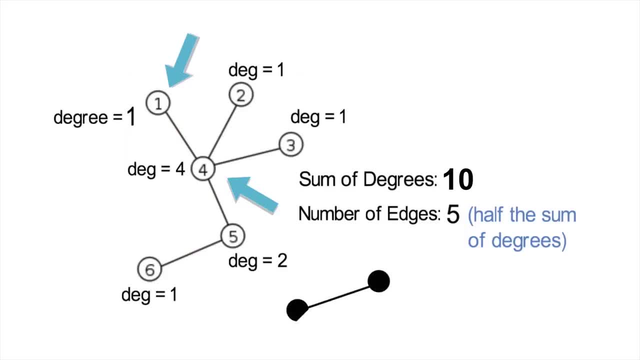 If we look closer, we'll see this is always the same number of edges or lines. If we look closer, we'll see this is always the same number of edges or lines. That's always true. Every edge connects 2 nodes, So that one edge makes both nodes have a degree of 1 for a total of 2.. 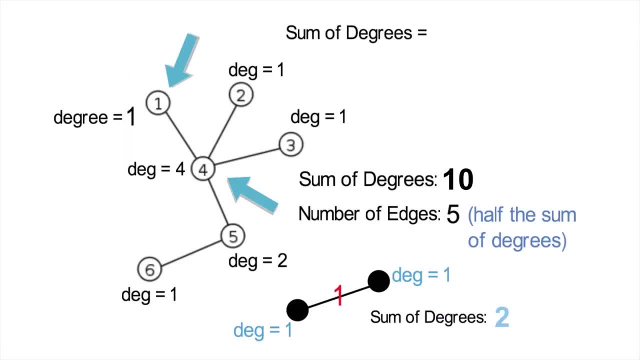 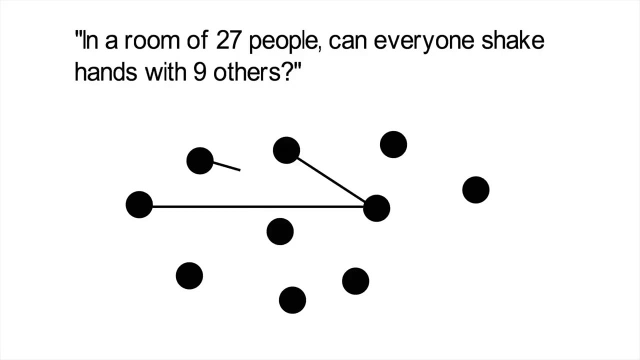 So we have something very important here. The sum of the degrees adding every single line that leaves each dot is always twice the amount of lines or edges that you see. Now we can go back to our problem. If everyone must shake hands with 9 others, then every node or dot needs 9 lines coming. 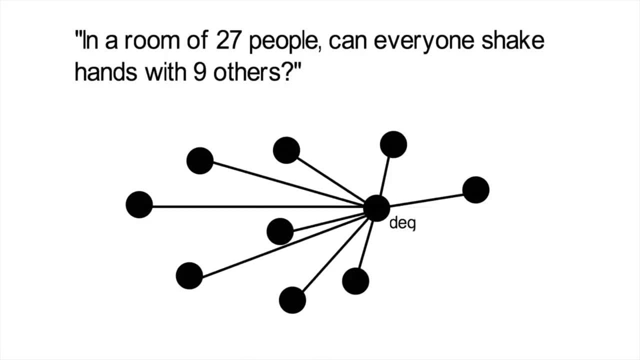 from it, meaning they gave 9 handshakes. Therefore every node would have a degree of 9.. If 27 nodes all have a degree of 9, then the sum of those degrees is 243.. And we said the sum of the degrees. 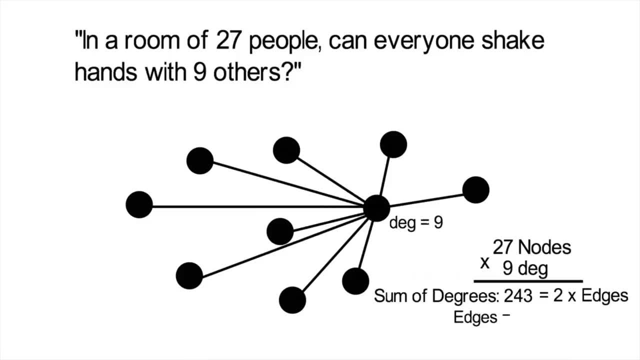 is always twice the amount of edges. That means there are 121.5 edges, which is not possible. The amount of edges or lines has to be an integer, like 1,, 2,, 103, et cetera. So the answer is no. 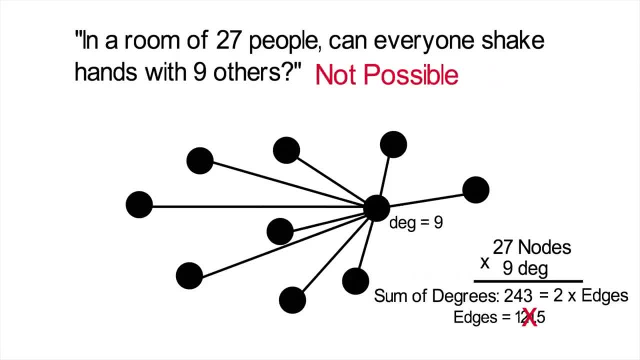 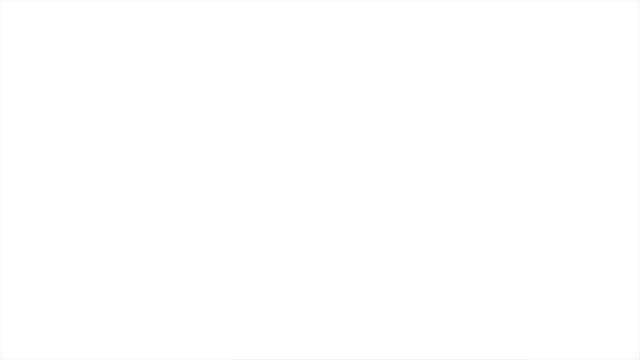 In a room of 27 people, everyone cannot shake hands with exactly nine others. If you did not get that, try this next one. If we have a bunch of nodes that represent locations, maybe cities, and edges which represent roads between them, 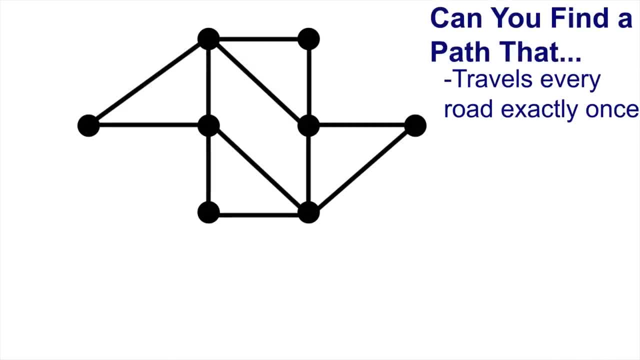 can you find a path that travels every road exactly one time and ends exactly where you began, So you can pick where you start and once you use a road, you can never use it again. I'll just tell you: the answer is yes. 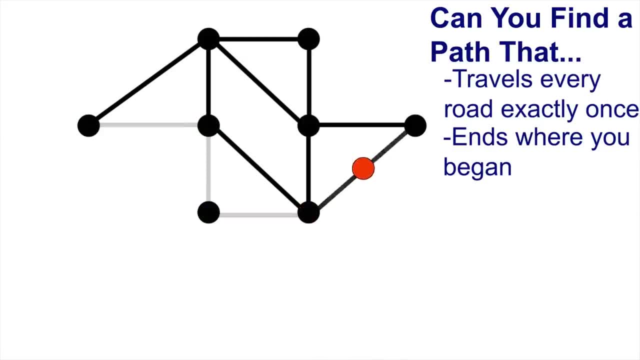 You can go to each city and use every road only once. There is more than one way to trace this path out, but this is one way to go over every edge only once and end up exactly where you started. This type of path is called an Euler tor. 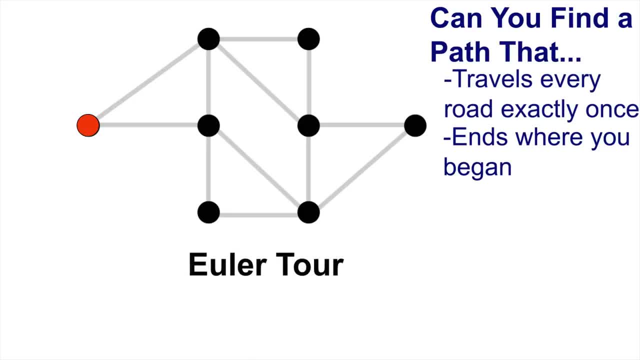 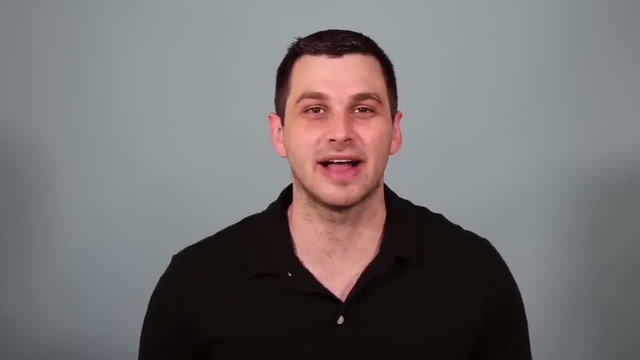 where no lines are repeated and you end where you started. Now real quick. this is sort of a side tangent and I don't know why I remember this, but when I was in high school, one day my friend challenged me in class to draw this shape. 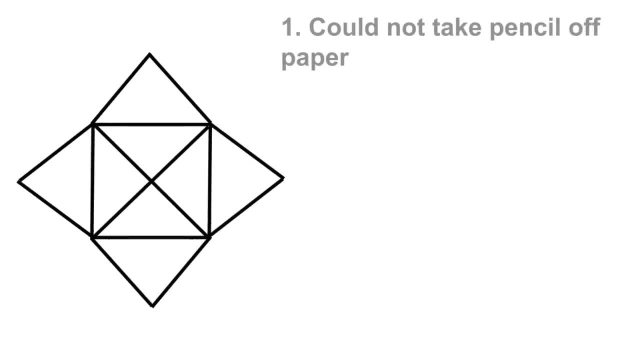 but with two conditions: I could not take my pencil off the paper and I couldn't do it, And I could not go over the same line twice. This was just randomly brought up, by the way. My friend probably heard it from another friend. 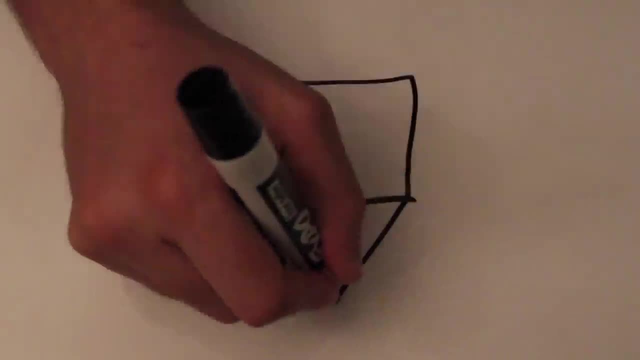 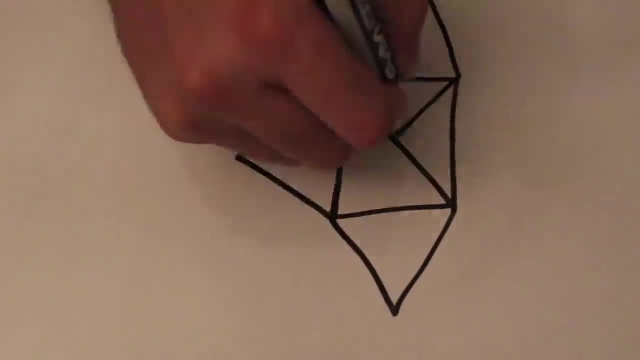 But no matter how many times I tried, I could not do it. I was always like one or two lines off but I could not complete it because it would require me to go over the same line twice. I think I remember this because I tried so many times. 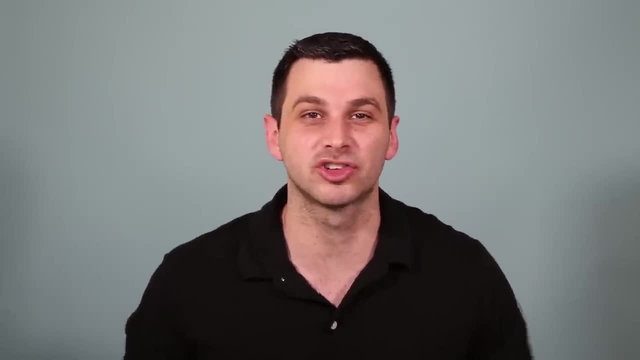 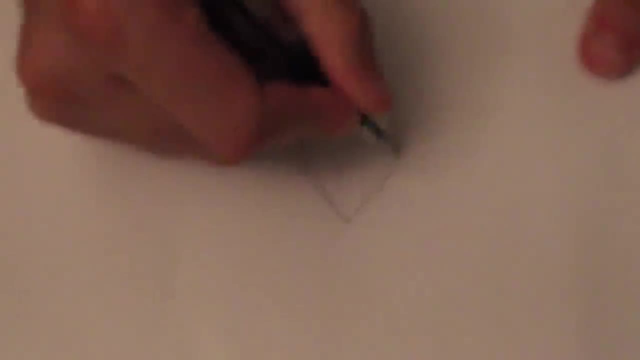 and it was bugging me. Neither of us knew whether it was impossible or we just couldn't find a way to do it. But years later, while learning graph theory, I read over this one theorem, then almost immediately took out a pencil and paper and drew the shape which: 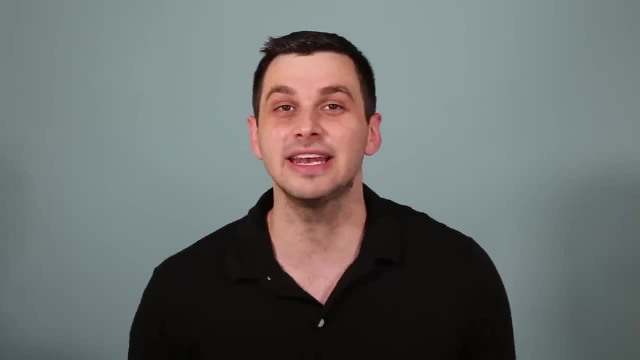 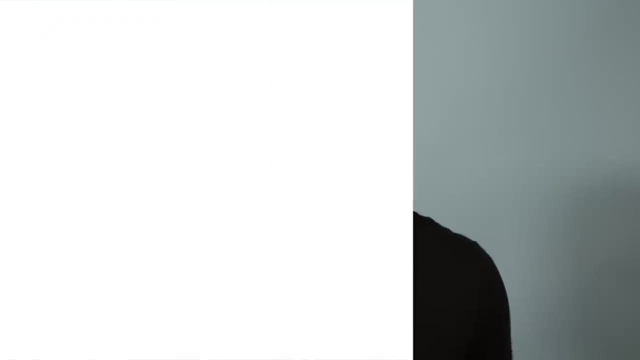 I still had in memory. I took a single look and realized finally, not only is it impossible to do, but I knew exactly why, and I want to explain that here. So why can we find a path here that goes to every city once? 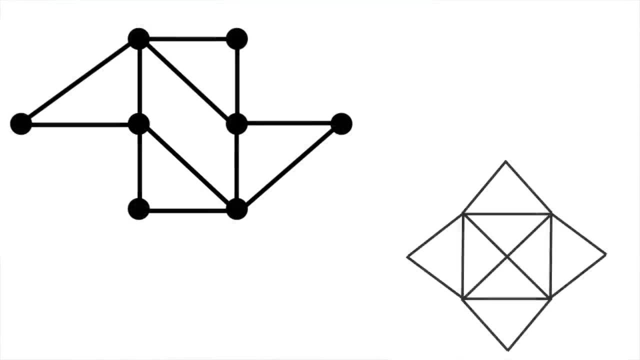 without reusing a road. but we cannot draw this shape without retracing a line. Well, on this graph that we can find a path for, we have to start somewhere. We then have to go to some node via some line or edge. 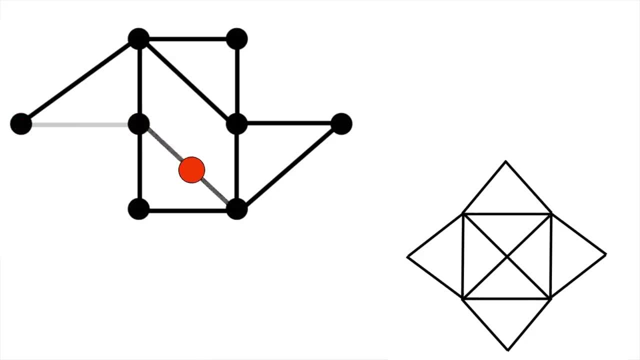 Then we have to leave that node and go to a second via a different line or edge. Every time we take one line to get to a node and another line to leave it, And if we ever return to that same node, it must be via a new line. 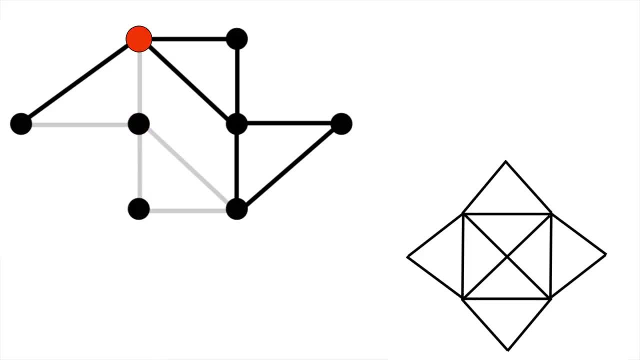 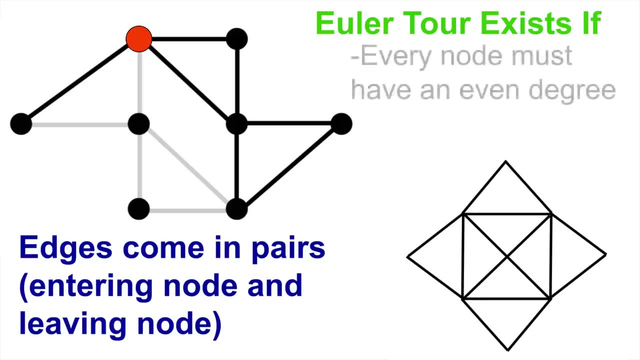 And we must leave via another new line. Notice, all of these come in pairs. So in order for an Euler tour to exist, such that we never repeat an edge, every node must have an even degree For every line that comes into a node. 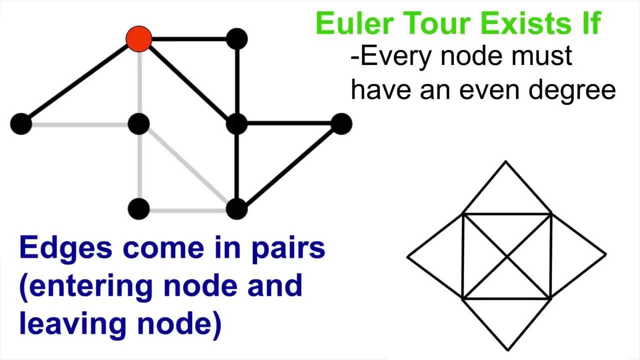 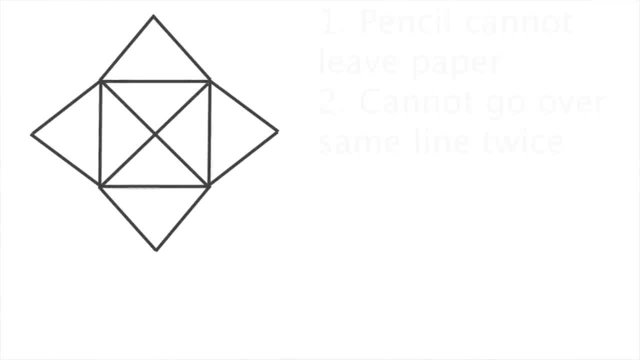 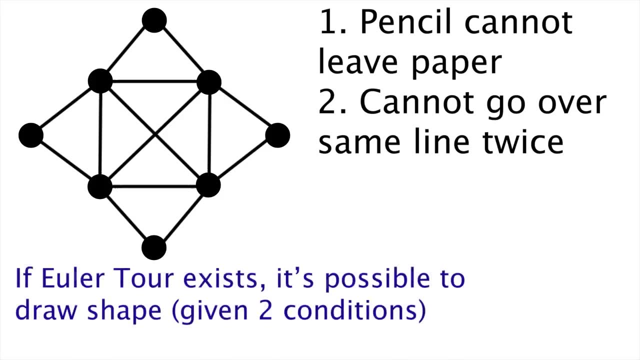 a different one needs to leave, Just like you see here. if you look at the degree for every node, they're all even Now going back to the drawing. given the two conditions, if we just represent these points as nodes, we can say that if an Euler tour exists, 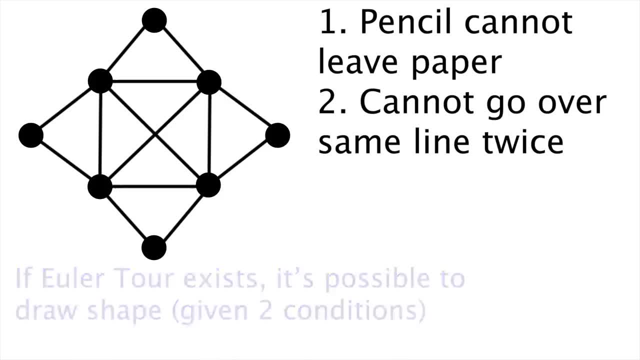 then it is possible to draw the shape. I mean, just take the last graph. You can think of the red dot as a pencil drawing it out. We know it won't go over any line twice and it never will leave the page. 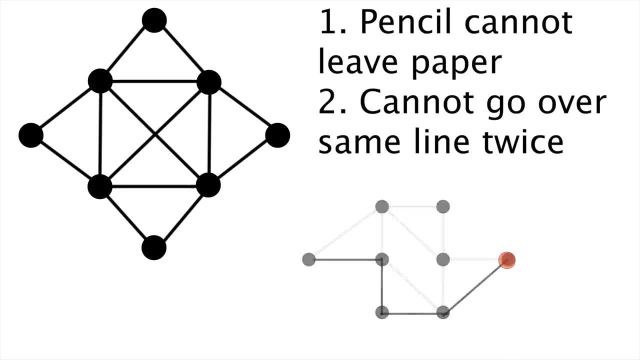 Therefore you could draw this graph, But in the drawing we have here the degree of these nodes is 5, because 5 edges leave them all And 5 is an odd number. So an Euler tour does not exist because all the nodes 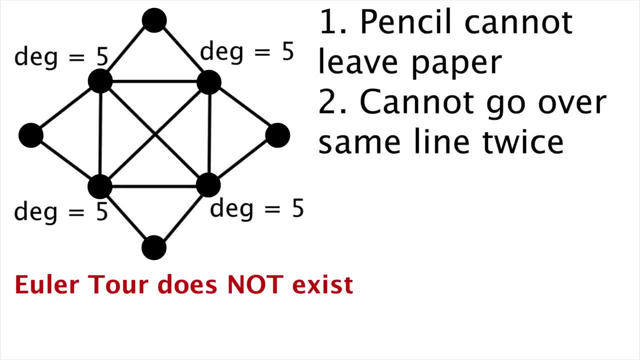 need an even degree. But we aren't even clear yet. Neither condition said that we had to end where we started. We can end wherever we want, We just can't go over the same edge twice. Now this is called an Euler walk. 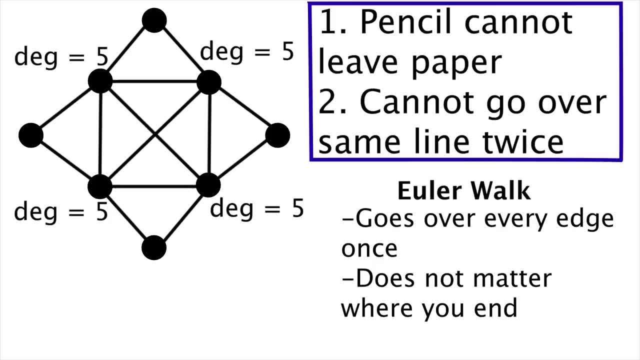 It's the same as an Euler tour, but you can end wherever you want. For example, this graph has an Euler walk. We can go over every edge just twice, edge just once, and we don't end up where we started. but that's totally fine. i won't show why. 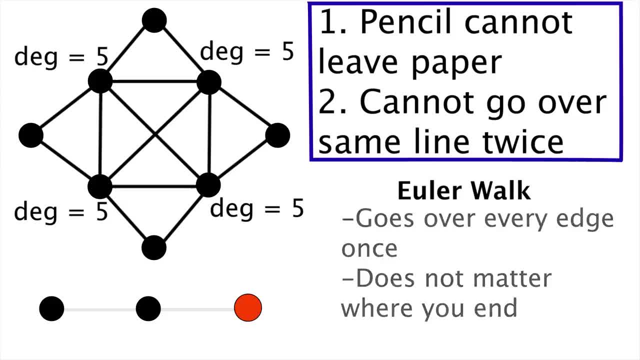 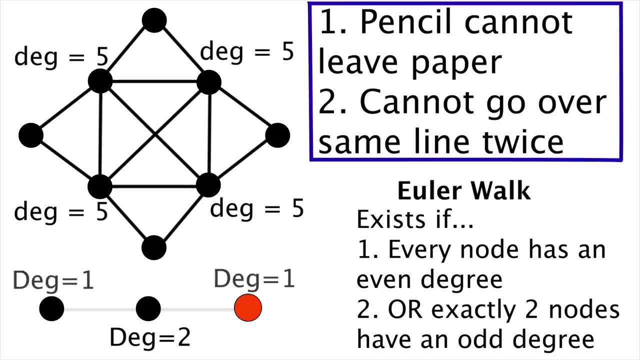 but you can prove fairly easily that, even though an oiler tour needs every node to have an even degree, an oiler walk will exist if, and only if, every node has an even degree or two nodes have an odd degree, like here: this node has an even degree, but these two have odd degrees. and since 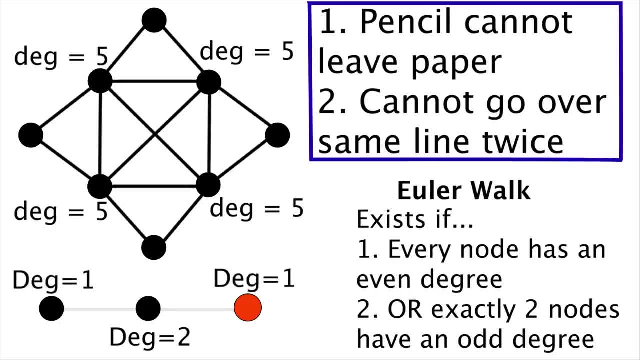 it's exactly two that have odd degrees. the criteria for an oiler walk is met. and now look back at our graph above. remember four of these nodes have an odd degree. therefore, an oiler walk does not exist. this means, if you think of the red dot as a pencil, we cannot go over every edge just 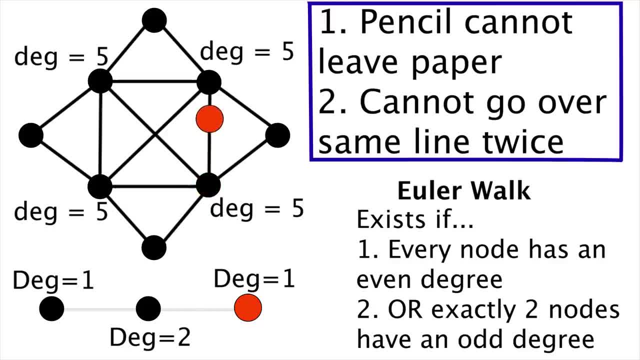 once without repeating. therefore, we of course cannot draw the shape without going back over a line, and that means this condition, that is basically saying an oiler walk must exist- cannot be met, and that's why i just possible to draw this shape given these two criteria. then one more quick graph theory. example has to do with cycles and trees. 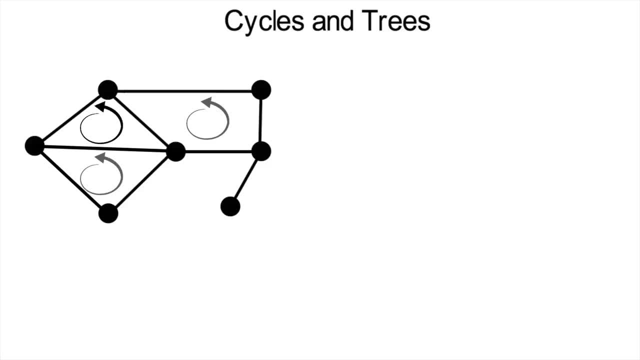 this graph right here has a cycle. in fact it has multiple. there's a way to start somewhere and trace some path where you end at the same place without repeating any nodes or edges. this graph here has no cycles, which means it's called a tree. here's something you'll prove in class as a computer scientist or mathematician. 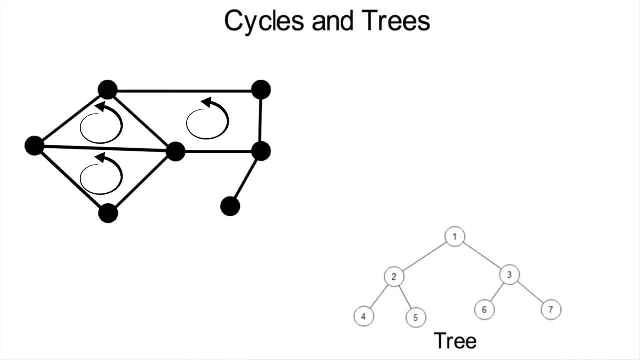 no matter what can connected graph you have or how many cycles it has, like this one above- there's a way to remove certain edges such that you have a tree but don't lose any nodes. they're all still there and everything is still connected. this is called a spanning tree. so imagine we have 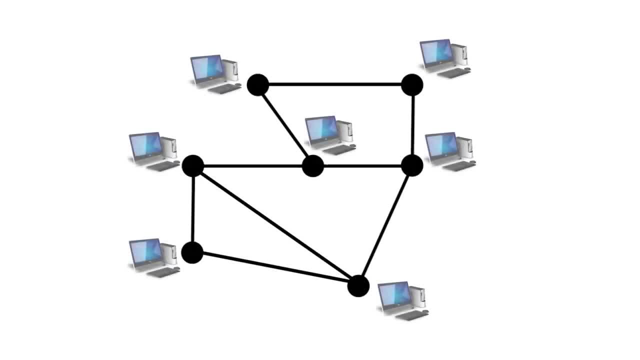 this graph where the nodes represent computers and the edges are long cables that connect them. maybe for some reason there's an issue where this network is too expensive with maintaining all the cables. maybe you want some way to keep all the computers connected but have the minimum amount.